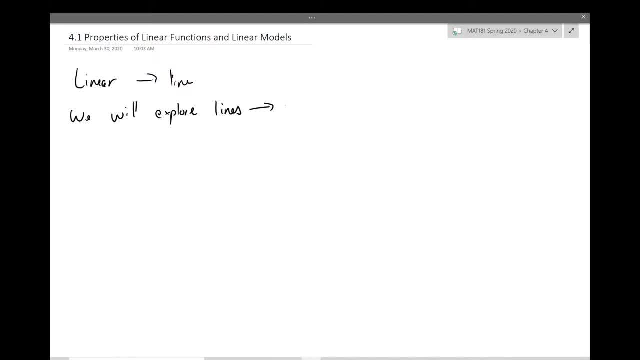 the thing that always comes with lines: Linear Models. Linear Models are two things actually. The first would be a slope and y-intercepts, and those are always important for us. First, let's define a linear function. A linear function is a function of the form f, of f, So we can just go ahead and do that. The first function, 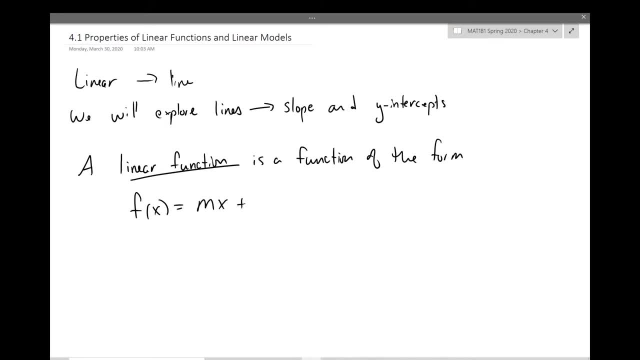 x equals mx plus b. all right, and this should kind of look a little similar to us, all right, because we know, remember this: y equals mx plus b. all right, remember, this is our slope intercept form. okay, and the only thing that we're really changing with this is the y is now abbreviated as f of x. 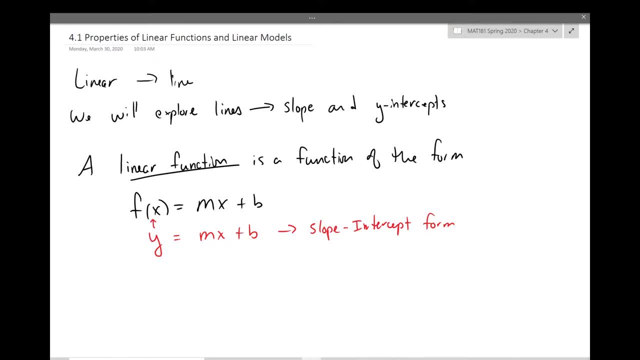 okay. and what's really nice about this about functions is- and you have to remember, with that function machine, okay, you have an input, then in this case it's going to be the mx plus b and then you're going to get an output. and if we have a function, functions allow us to predict. 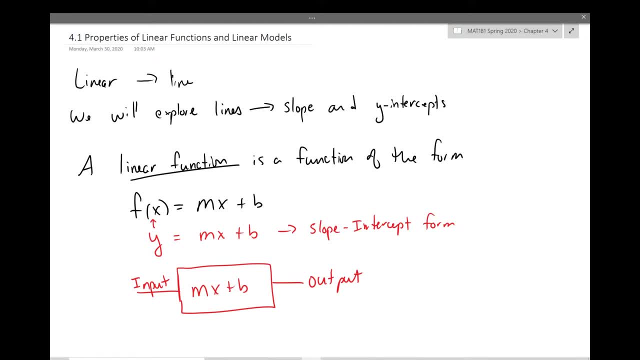 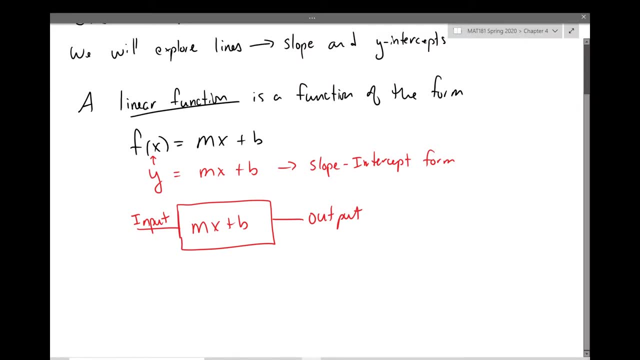 things. okay. functions allow us to predict outputs given a certain input. okay. so let's just finish this up, this definition here. so let's see here: a linear function is a function of the form f of x equals mx plus b, and m will be our slope and zero comma. b is the y- let me write that nicer- here is the y intercepts, okay. 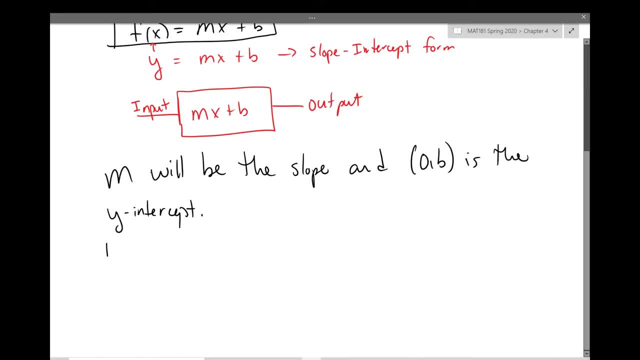 all right. um, just i'm going to throw this in here: our domain is the set of all real numbers. now remember domain. all right, domain are x values. okay, and another way to say x values it would be inputs. so when we have a linear function and we're using the function machine, we're 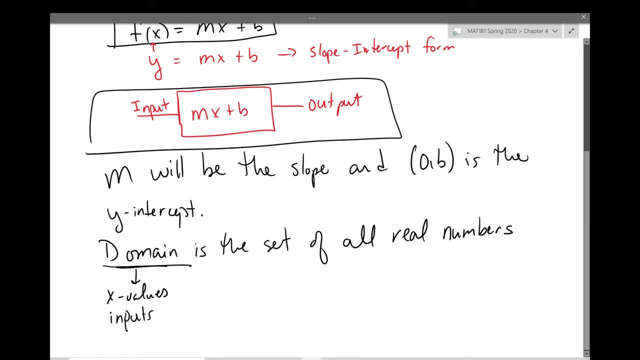 going to use the function machine right here that i just uh boxed in we have. if we have a linear function, i can use any x value in the real numbering system, because i'm always going to get an output. okay, because all linear functions. well, i- how about i say it like this- all linear equations. when 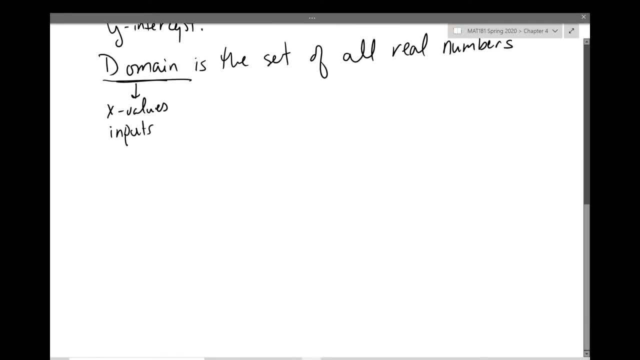 graphed are functions. okay, so let's go ahead. let's look at an example here. let's graph a linear function, so graph a linear function. okay, all right. so let's see um graph f of x equals negative 3x plus 7 and state the domain: okay, so for us this is going to be, uh, relatively simple. 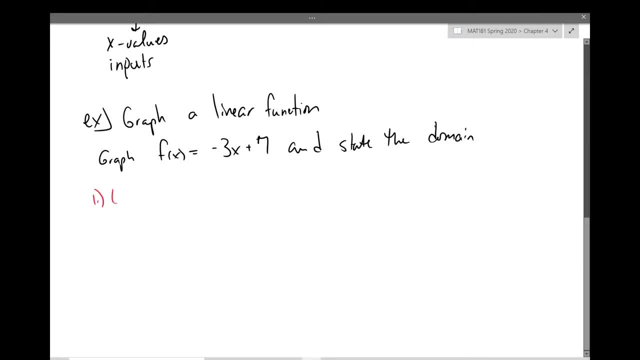 first let's label. sorry i'm i. i'm just writing for the first time today, so it's gonna be a little sloppy initially. so first label the slope. all right, so our slope is right here. it's the coefficient of the x, very or x term. so slope is negative three or m equals negative three and then two. 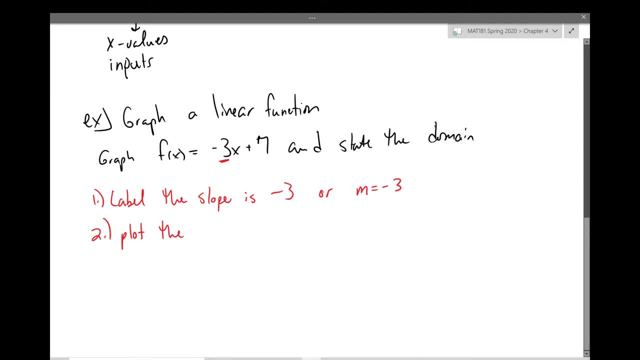 so slope is negative three, or m equals negative three, and then two. plot the y intercept. so our y intercept is going to be zero comma and in this case- let's highlight it here- it's that value right there. okay, so this is going to be zero comma, positive seven. 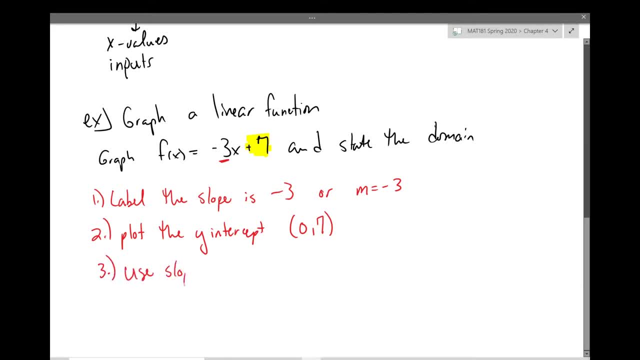 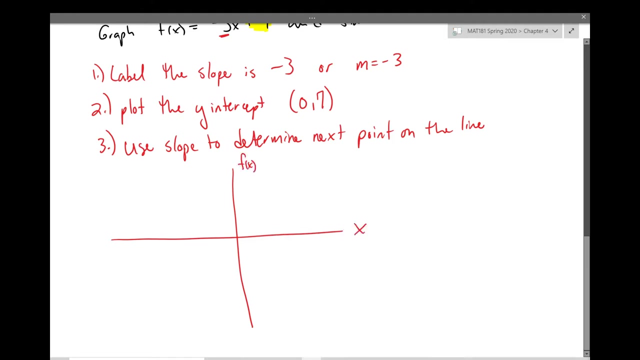 and then three use slope to determine, and on top of right here it's going to be exactly what you see on the computer at the i. oh yeah, it is that dynamic value widespread. okay, so this is what we call the y-axis. okay, so basically, let's pull people up and and raise them up that time. 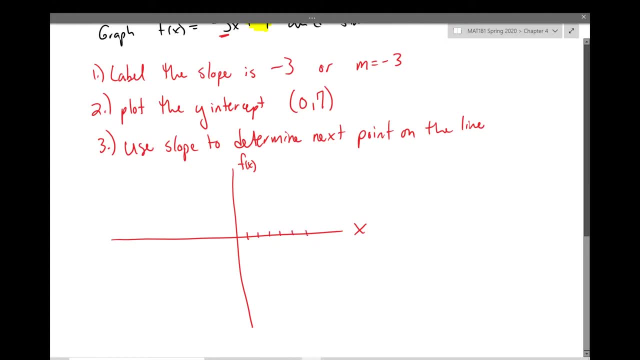 take it to f and on the y-axis i'm gonna put a test to see how bad it is. i would want to know what set the same value is that? that might be a zero or three levels. each regular function thing to use would be some sort of graph paper. uh, clearly i don't have that, because i'm writing. 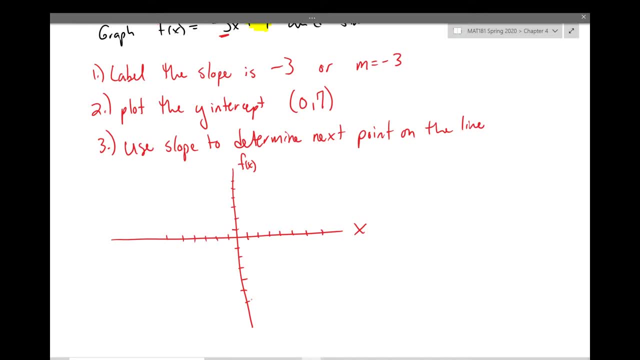 on my laptop. so you know i do what i can. so, uh, let's see here: zero comma seven. so that's gonna be one, two, three, four, five, six, seven. so that's right here, all right, and i'm gonna label the point. put a little arrow: zero comma seven. now i use my slope to determine the next point. since my slope, 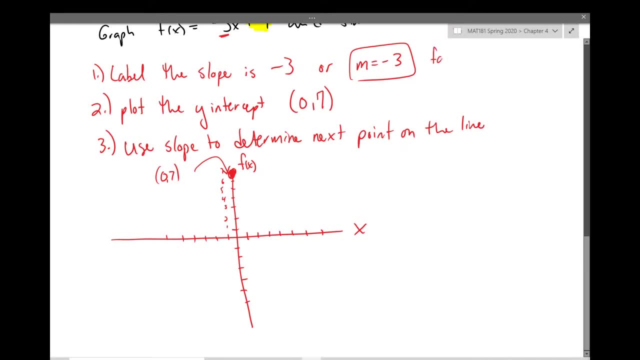 is negative three. i know i am falling and then moving to the right. okay, so falling to the right three. so i'm sorry, falling down, falling three to the right one. so, starting at zero comma seven, i go down three units. so that's going to be one, two, three, so it's right here, and then i go over one. 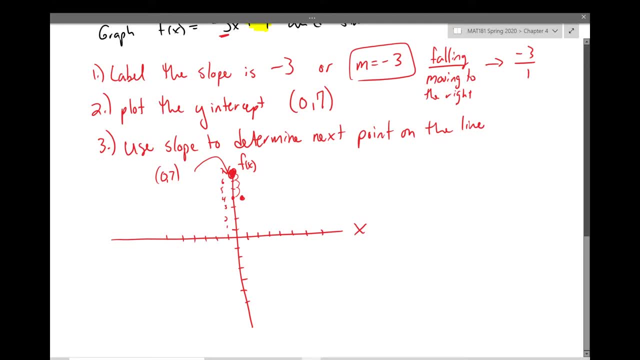 and there's my new point. so let me get rid of all this other stuff here. all right, so one, two, three to the right one, there's my point, and i just connect the dots. that's it. now i need to state the domain. well, remember, since, uh, since we have a linear function, my domain. 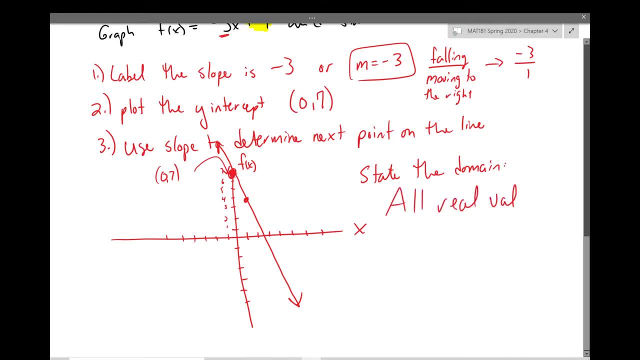 all real. i don't want to say values, let's say all real numbers. another way to say this is just to label it. the domain goes from negative infinity to positive infinity, all right. now let's take this concept of slope, okay, and and linear functions, all right. 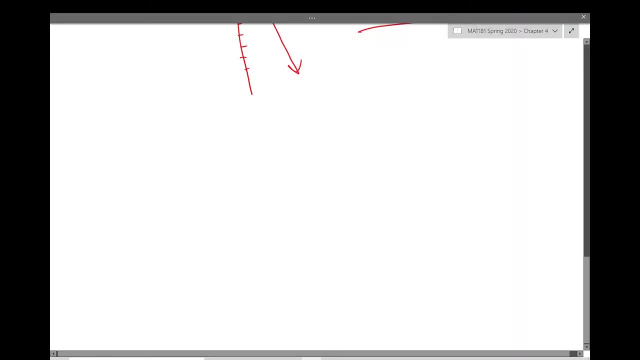 and what i mean by that is this: when we are talking about slope, okay, we know- or we we've explored this already in class- we know slope m is equal to the negative draws two, and that's okay. we know slope m is equal to the level of the final point, which is the number of points, okay, and then we're going to talk about that in just a moment now. so what we're going to do here is to use the graph view. so if you're interested to learn this technique here, to learn this technique, 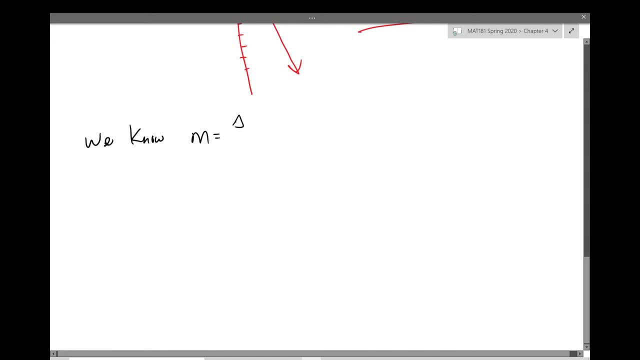 okay, and what i mean by that is this: when we're talking about slope, okay, we know, or we, we've explored this already in class- we know slope m is equal to the change in y over the change in x. right now, a way to another way to. 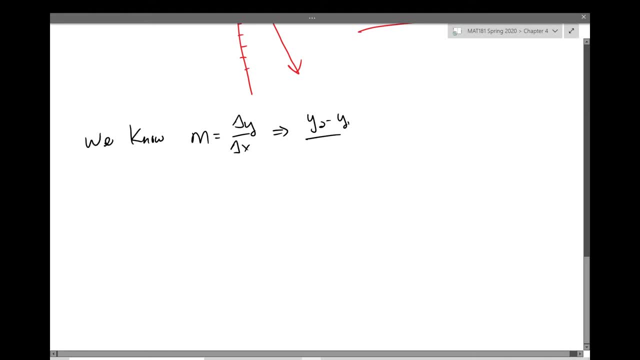 write that is y2 minus y1, all over x2 minus x1. okay, and what we are really finding here? okay? another way to describe slope is to call it the average rate of change. okay, so our average rate of change, which I'll abbreviate as arc average rate of change, is slope. okay, like so when you 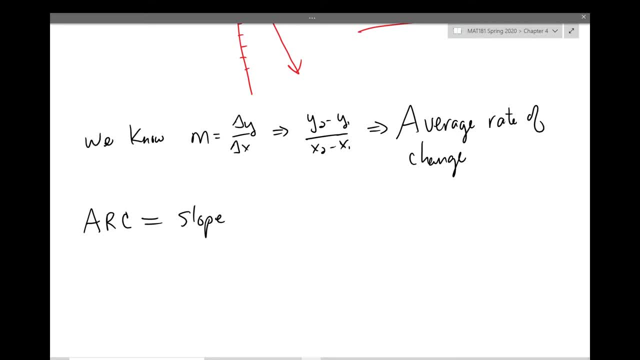 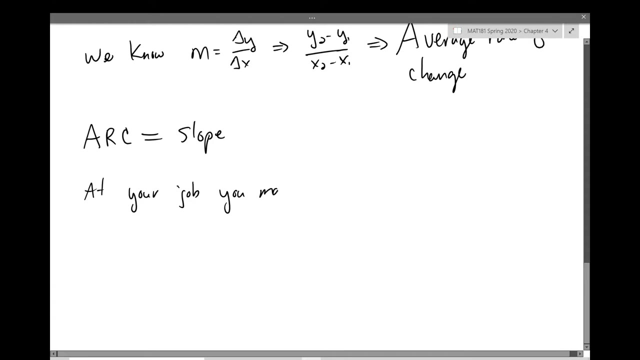 think about it. um, when you are working, okay, let's say you're at your job- and I know I use this example a lot in class- all right, So let's say you're at your job, okay, And you make at your job. you make $10 per hour, okay, Well, another. 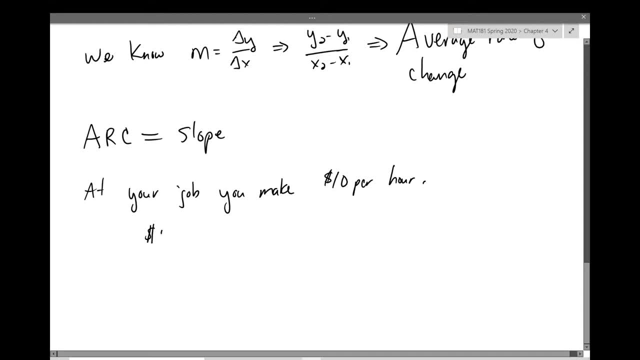 way to write this mathematically is $10 per one hour And you can see here that your average rate of change- on average, you will make $10 per hour, okay, So when we talk about slope, the other thing that needs to just start ringing off in your head is: oh, slope is the average rate of change. 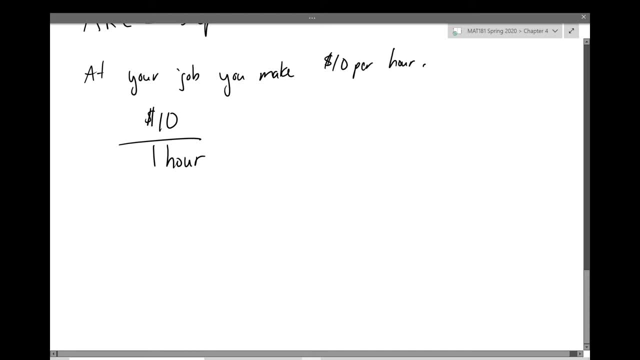 okay, And there are four types of slopes. remember four types of slopes And we've studied this already. I'm just reviewing. Okay, we have positive slopes, And remember, we read left to right- Oh, that's a horrible looking way to write F or left, Left to right. So here's a positive slope. 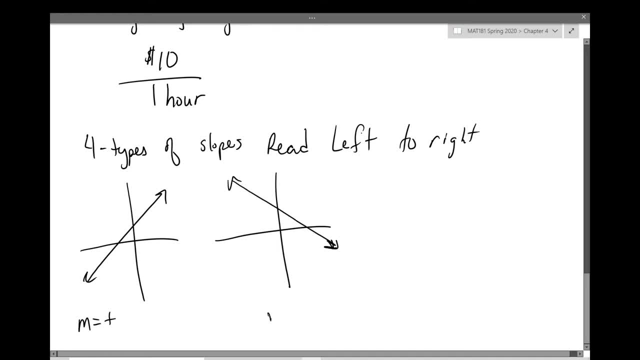 Here's a negative slope. Now here are the two fancy ones. okay, We have a slope of zero because it's a horizontal line, And then the last one slope is undefined. And it's undefined because X1 is not allowed to equal X2, okay, So let's look at, let's see if we can determine. 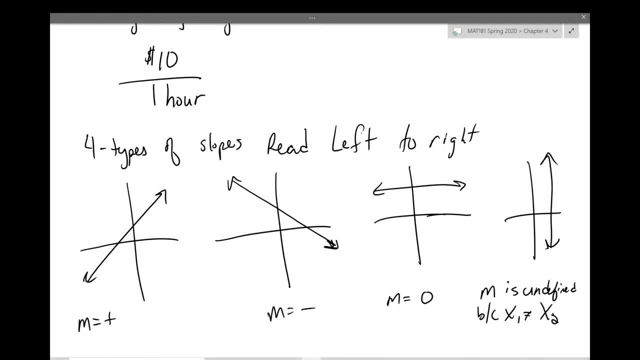 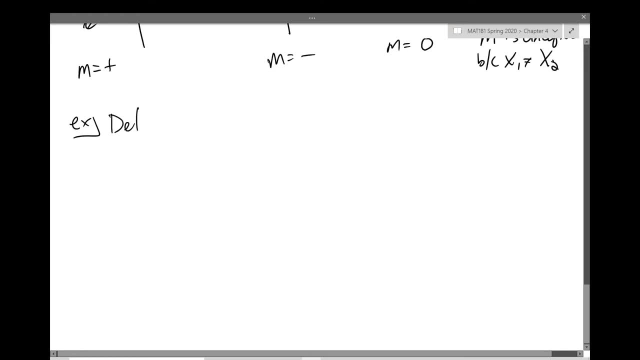 when we have a slope that is increasing, decreasing or constant. all right, So example here determine whether a linear function is increasing, decreasing or is constant. okay, So let's look at the first one here. Change my marker here. Part A F of X equals 5X minus 2.. All right, well. 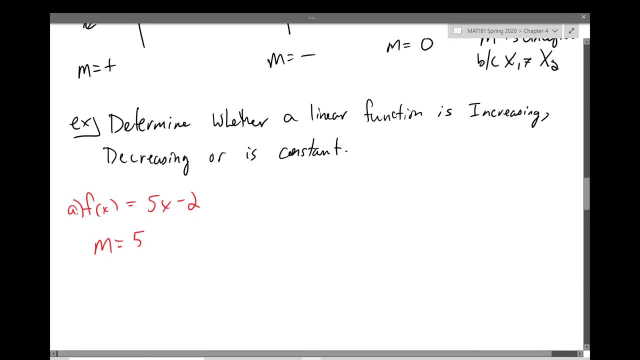 all you have to do is label the slope M equals 5.. Since M is 5, since M equals 5, and 5 is positive, our linear function is increasing. okay, That's how easy it is. Let's do another one real fast. We'll do a couple more. 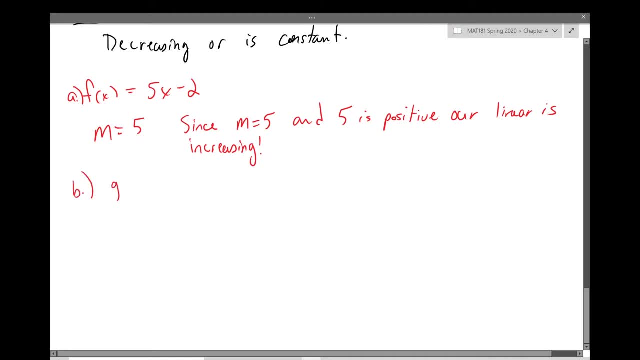 How about? how about B? Let's say, G of X equals negative 2X plus 8. Well, M equals negative 2.. So since M equals negative 2, and I guess negative 2 is negative, it's kind of redundant. 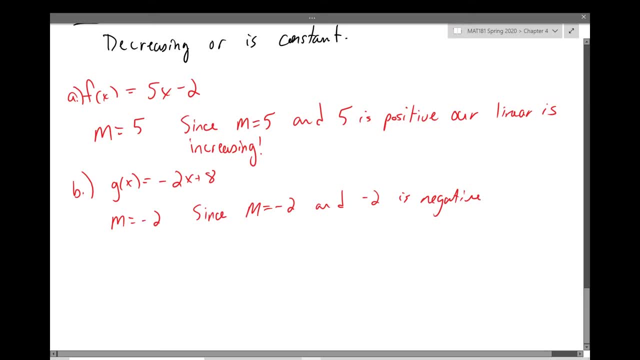 but I'm just, you know, keeping to consistency here. So since the slope is negative 2, and negative 2 is negative, our linear function is decreasing. okay, And I forgot to write the word function up here. Let's put that up there. Some of you will go into the comments and grill. 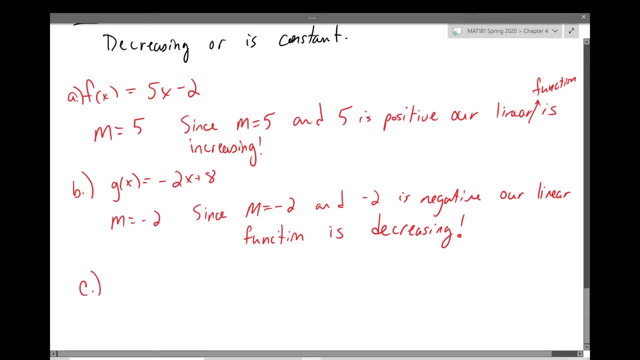 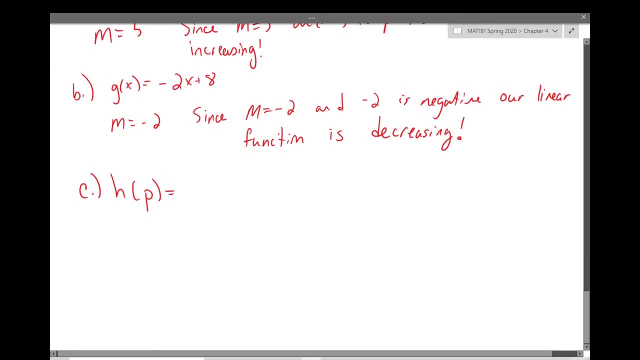 me for that. all right, Now how about this one? H of P equals 5.. Now, let's use a different number. How about 7,? all right, So H of P equals 7.. Well, you have to remember that we are dealing with linear functions. okay, And the H of P. 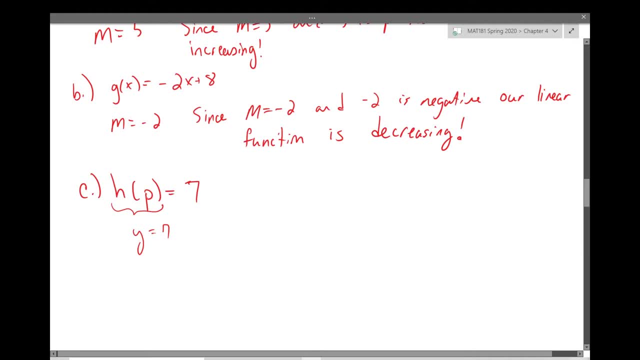 that we really think of that as just Y. So here, H of P equals 7 is the same exact thing as saying Y equals 7.. Now, if I graph, Y equals 7,, 1,, 2,, 3,, 4,, 5,, 6, 7.. If I graph that, notice it is a horizontal line. 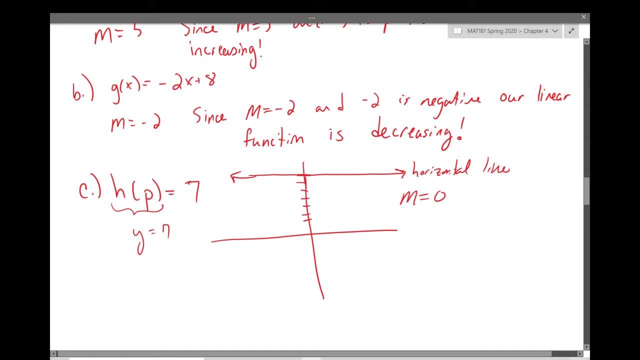 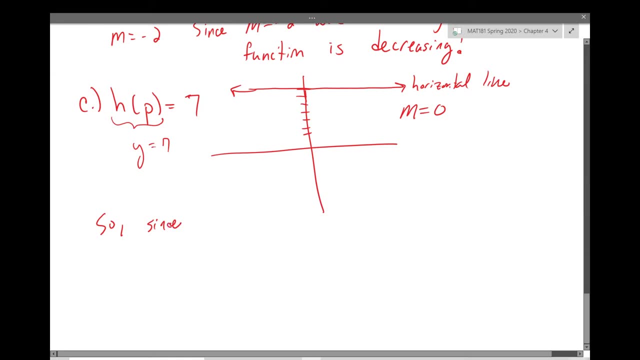 And all horizontal lines will have a slope equal to 0. So since H of P equals, 7 is A, we're agreeing that we have a slope equal to a 0 here. So in total, our sum of all side prêt dot. 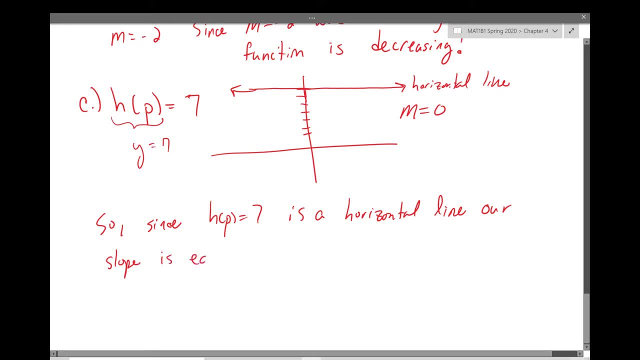 our slope is constant. Observe this So. So what happens is when you're rendering the. this is my diagonalrid. this is a imaginary linear function where the summer 16 goes down like this, or the weather side, the takeoff, goes down like this: 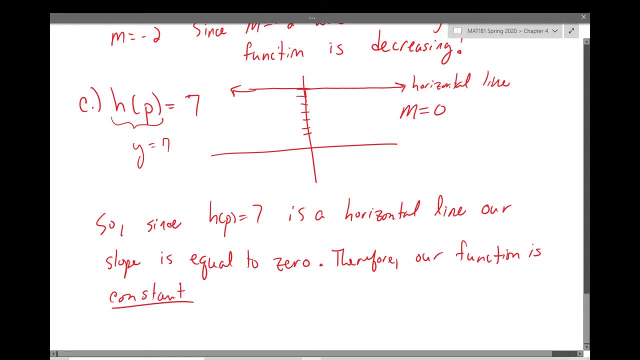 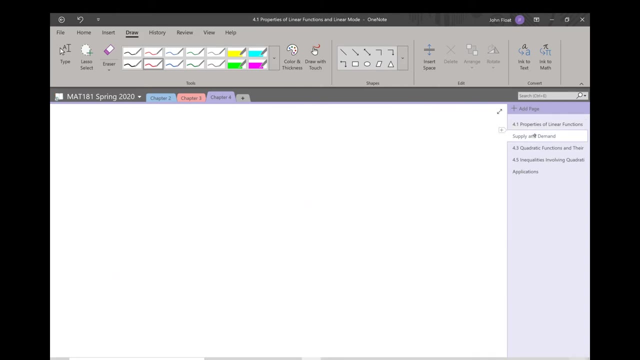 it's. it's a horizontal line and that that's as hard as it gets. it's. it's just being able to recognize what you know, what is given in front of you. okay, so let's talk about a very specific example here. all right now. I should have, should have it right here. there we go. 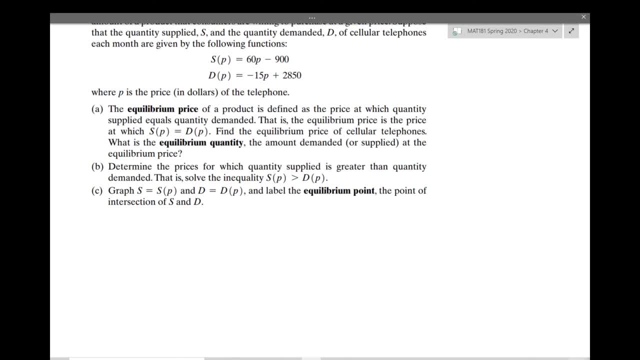 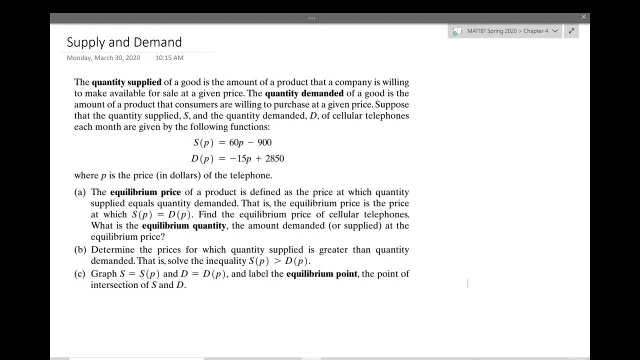 all right. so we're gonna talk about a very specific example now. this is our application. all right now, before we even really dive down and read all the fine print and everything, I just want you to look at these two equations. notice both. let me write it like this: notice that P is raised to the first power in. 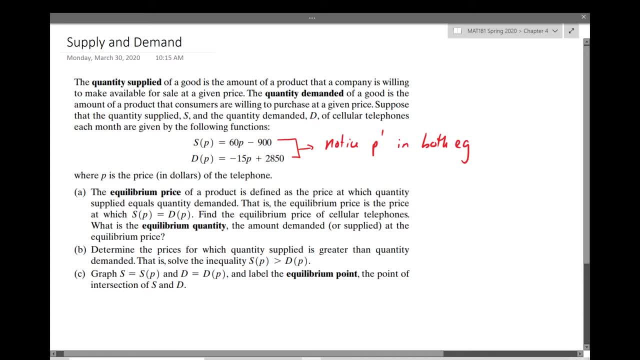 both equations. okay, so P is raised to the first power in both equations, which means linear. okay, all right, so let's go ahead, let's read it and let's decipher all this information. there's three parts here that they want us to answer, and that's fine, we can. we can go ahead and. 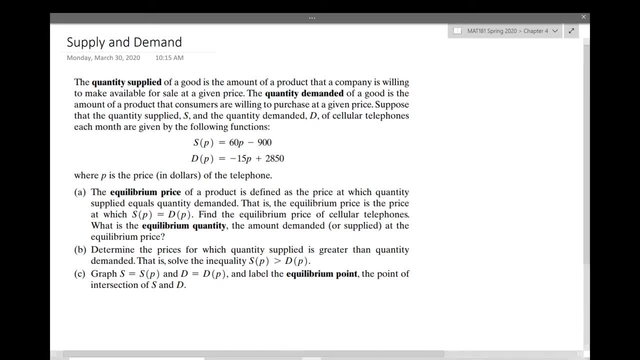 do this. so, first, the quantity supplied of a good is the amount of a product that a company is willing to make available for a for sale at a given price. the quantity demanded- I'll be good is the amount of a product that consumers are willing to purchase at a given price. all right, so the S of P. 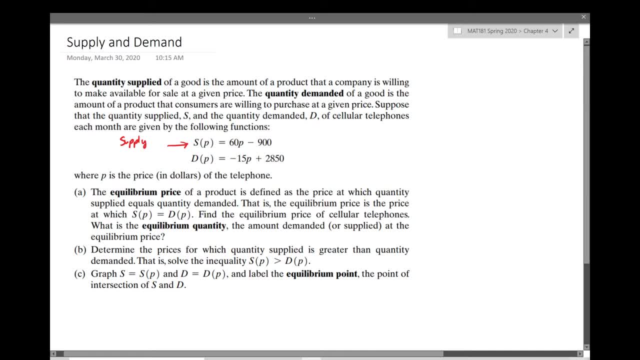 right here, that's our supply all right. and the D of P, that's our demand all right. so let's try this out. okay, here's our demand. okay, so let's see here. suppose that the quantity supplied s and the quantity demanded d of cellular telephones each month are given from the following functions: alright, so we have. 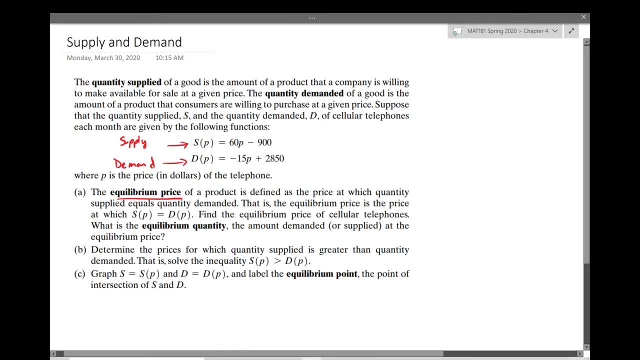 two functions: the supply function and the demand function. they want us to first find the equilibrium price in dollars of the cell phones. okay, now the thing you equilibrium price, the key, the root word is equal. Okay, So, uh, to find equilibrium price. 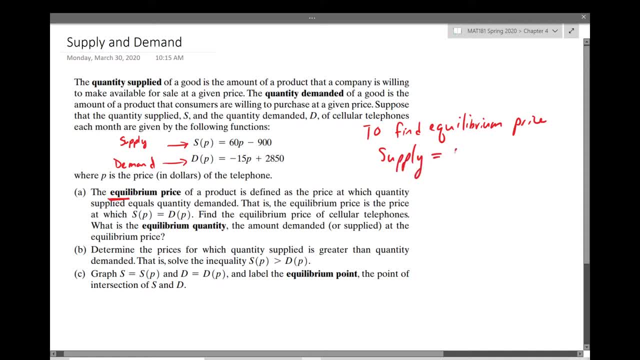 All right, Supply has the equal demand. Okay, Um, you can kind of think of this in terms of like profits. Okay, We know that. um, if you, if you, um, if you're making money, that means that. 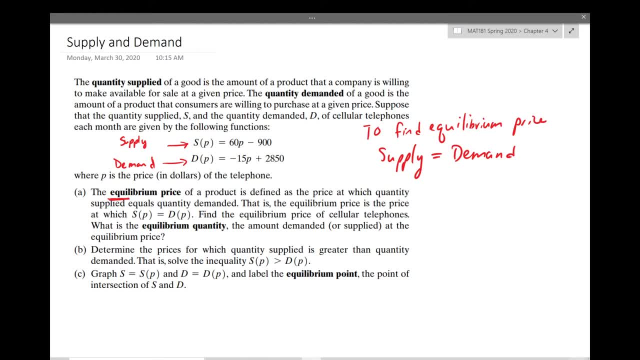 the revenue is exceeding the cost. If you're losing money, that means the cost is exceeding the revenue. Uh, or if cost equals revenue, then you were at that break-even point. This is: this is almost the same type of application. Uh, mathematically it's the same. You were looking. 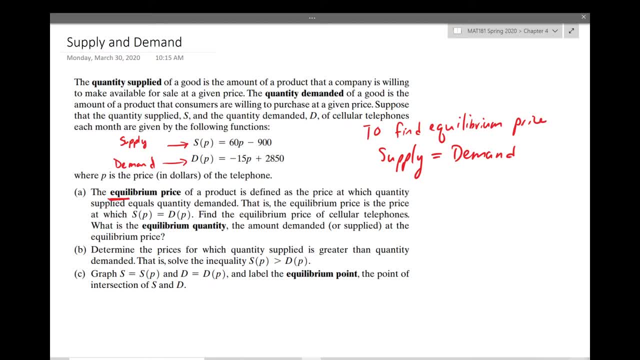 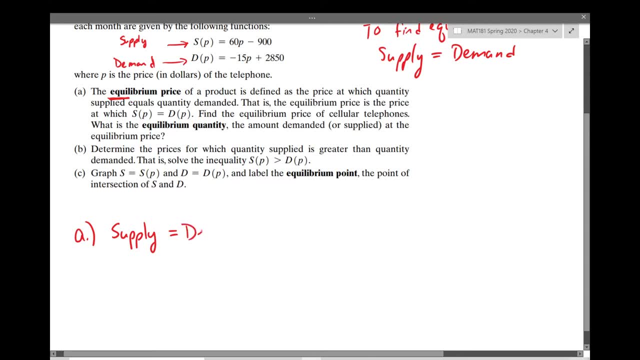 at an equilibrium. So you have to set the two equations equal to each other. So for part a, that's what we're Going to do: We're just going to set supply equal to demand. That's it. So our supply equation is: 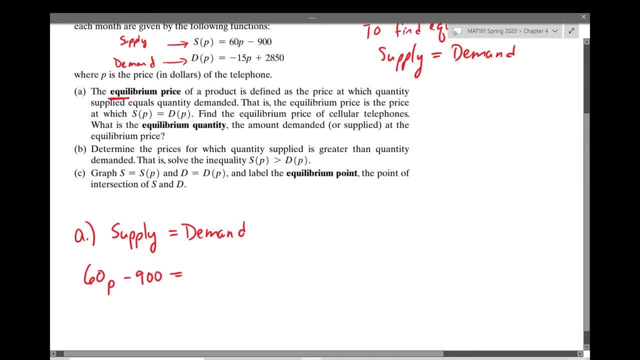 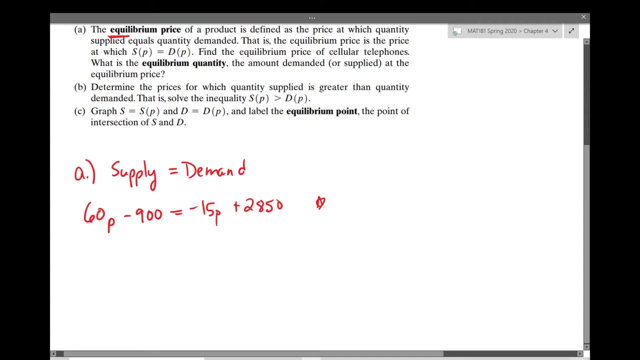 60 P minus 900.. Our demand equation is negative: 15 P plus 2,850.. Okay, And all we're going to do here- if I could spell that'd be great: Solve for P. Okay, So, let's go ahead, Let's solve for P. So, um, I'm going to add 15 P to both sides. 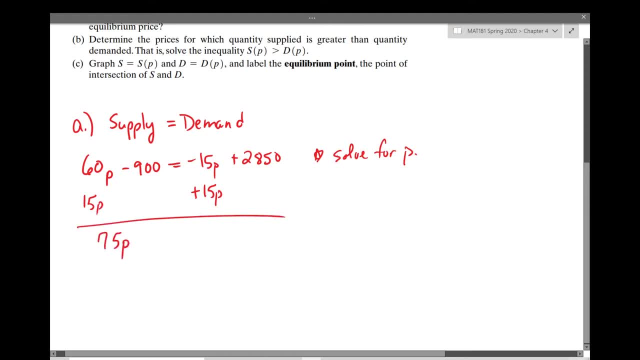 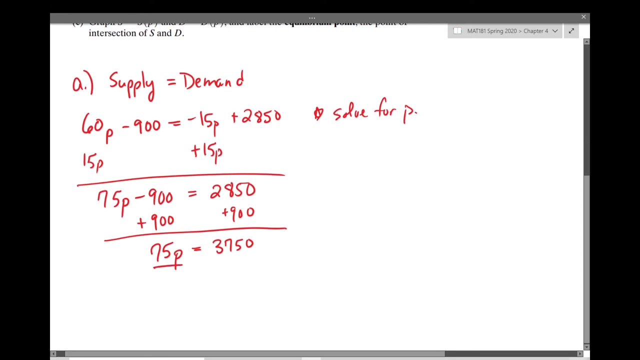 All right. So that's going to give me 75 P minus 900 equals 2,850.. Now I'm going to add 900 to both sides, So that's going to give me 75 P equals 3,750.. And then I'm going to divide both sides by the coefficient of the variable term. 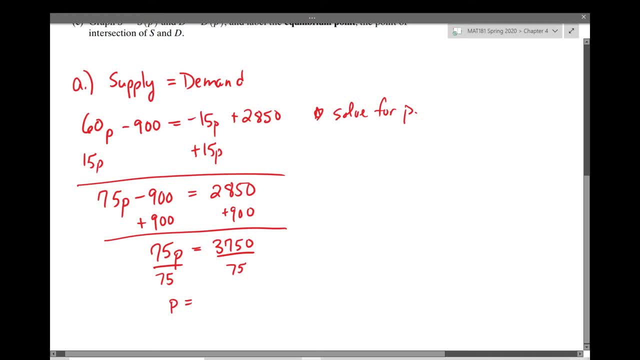 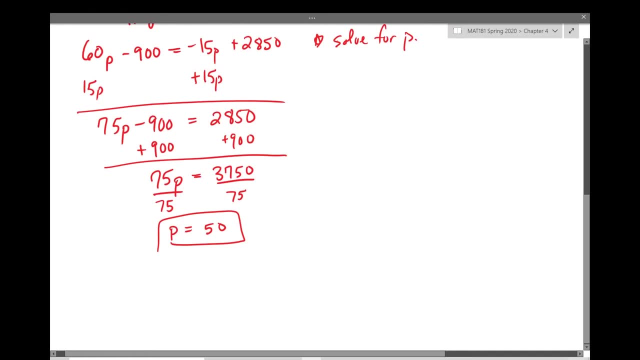 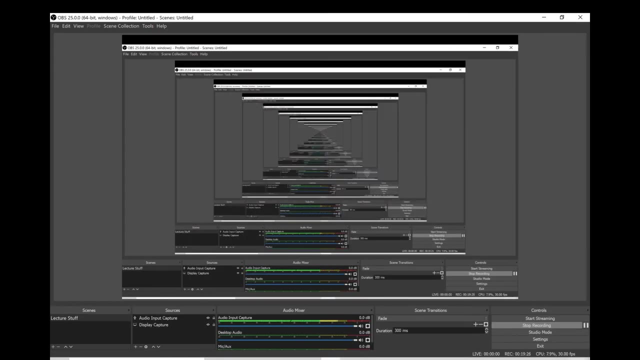 which is 75, to give me, P equals 50.. Okay, So the equilibrium now. we always want to. we always want to, you know, wrap this up with a nice sentence: Oh, sorry about that. Um, this thing right here that you just saw, this crazy looking thing. That's how I record my lectures. 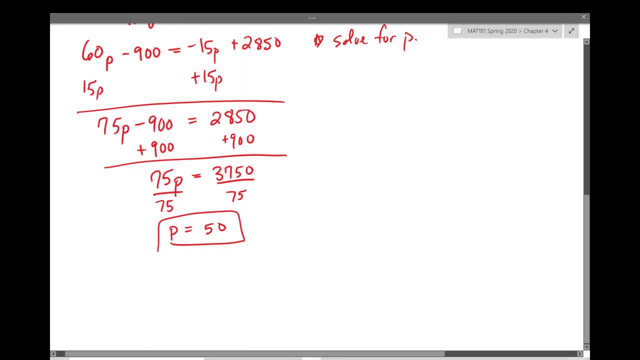 That's all. It's called OBS, It's a. it's a pretty powerful screen capturing Software. It's free, which is awesome, All right, So let's go ahead, Let's. let's finish this with a sentence: The equilibrium price. 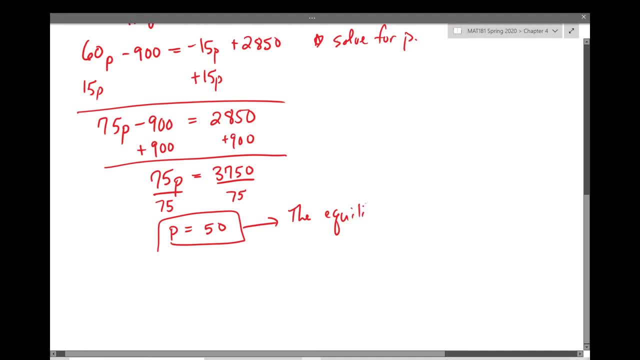 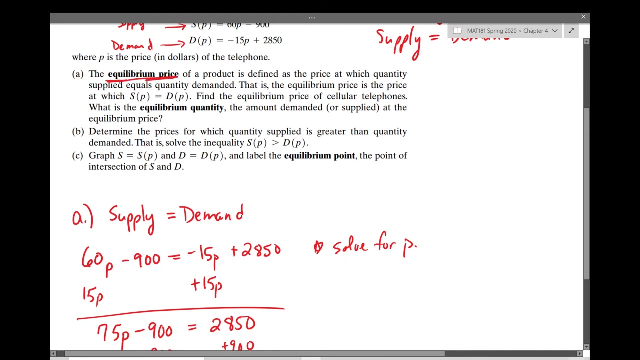 is $50 per cell phone. Okay, So to find the equilibrium quantity, all right, because that's the second part. they want, Remember, they want us to find the equilibrium price. uh, that is okay. Uh, and then fine, based from the equilibrium. 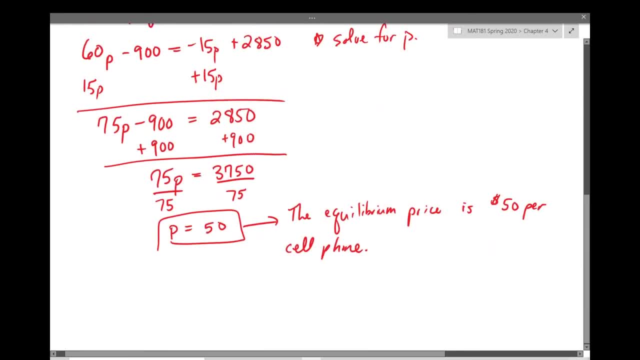 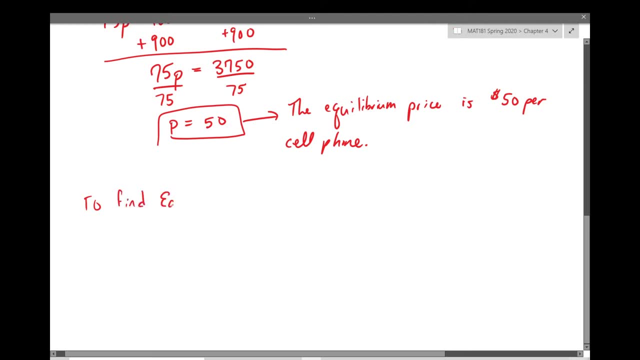 price. what is the equilibrium quantity? All right, So to find that equilibrium quantity, I'm going to abbreviate equilibrium with just EQ, equilibrium quantity which is used. the fact that we that we know P equals 50 and we substitute into D of P equals negative 15, P plus 2,850.. Okay So, 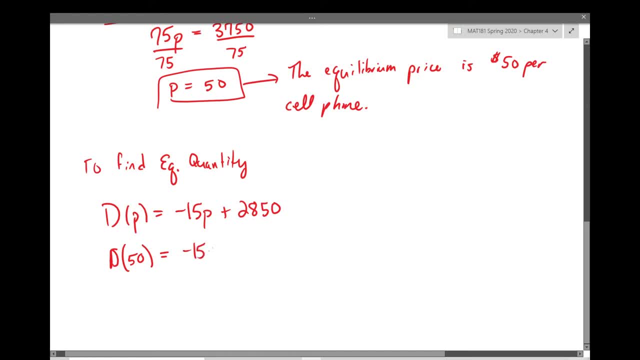 D of 50 equals negative 15 times 50 plus 2,850.. So I'm going to go ahead and, uh, I'm going to just calculate it real fast. Hopefully you didn't hear it earlier when I was hitting the buttons. 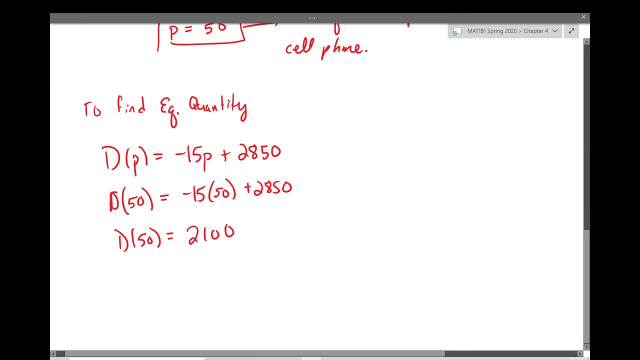 So we need 2,100 phones, cellular telephones. So at a price point of $50, the demand- let's write it like that- The demand will be 2,100 cell phones. Okay, All right, So let's look at what part B says. All right, So let 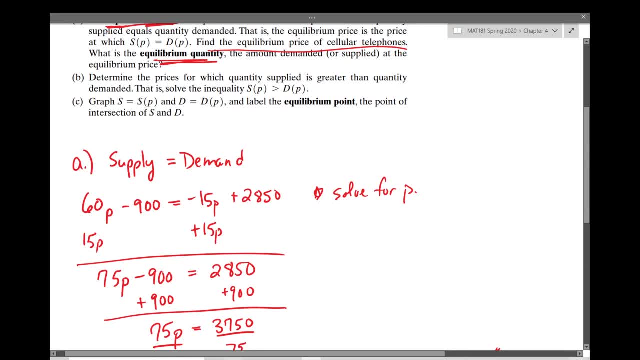 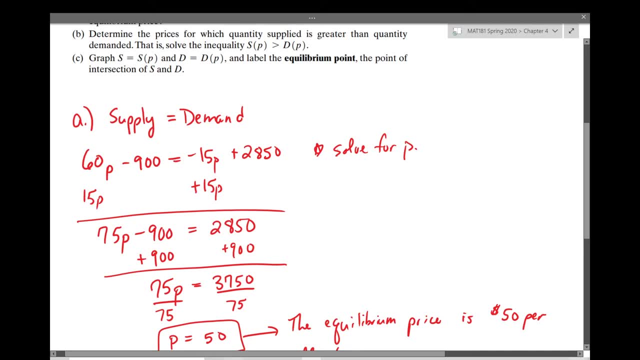 me. uh, just do a little part B, I'll scroll back up And if you need to, you can always pause the video and stuff like that just to read it for yourself. So, uh, determine the prices for which the quantity supplied is greater than the quality demanded, That is, solve this equation right here. 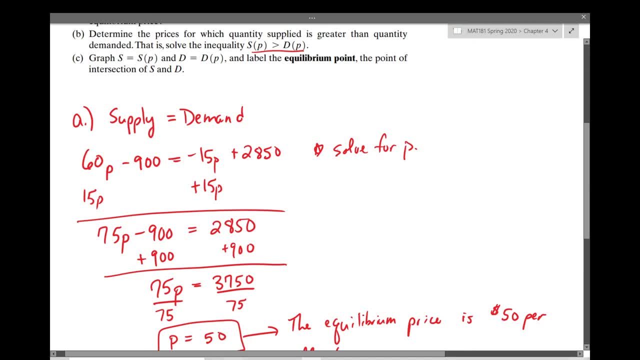 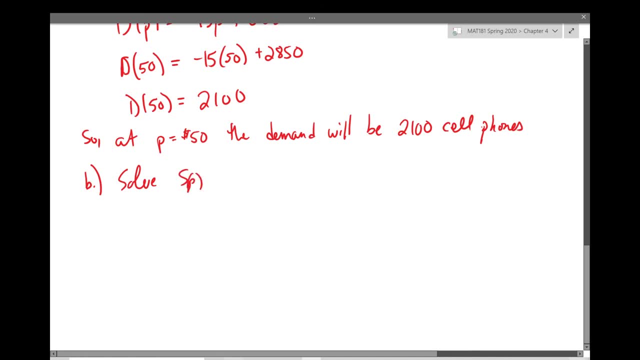 All right, That's fine, We can. we can do that. do that. So S of P is greater than D of P. So solve S of P. let's write that cleaner is greater than D of P. All right, So that shouldn't be too difficult. Once again, we 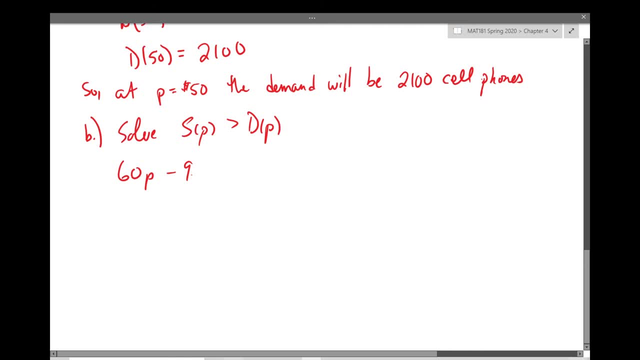 set the supply, 60P minus 900, is greater than negative 15P plus 2850.. And if we go ahead and we do our math again, so I'm going to add 900 to both sides, That gives me 60P is. 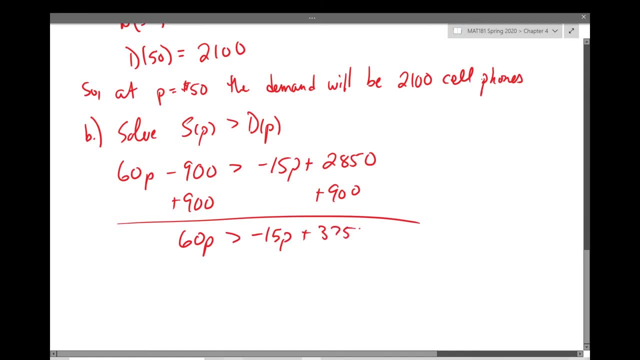 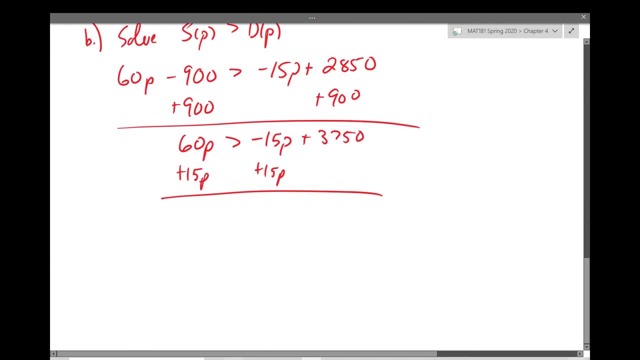 greater than negative 15P plus 3750.. Add 15P to both sides, That's going to give me 75P. It's greater than 3750.. And then, last but not least, divide both sides by 75.. All right, We have. P is greater than 50.. Now remember, the key is: 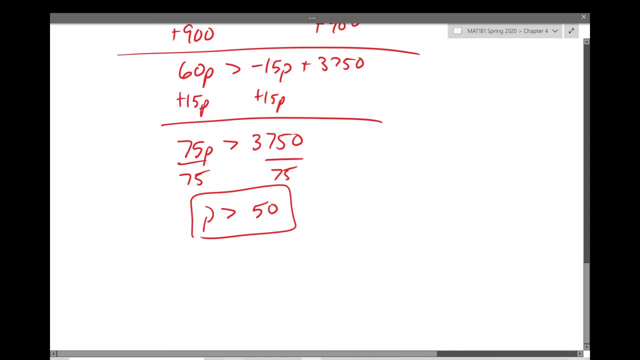 to give me an interpretation what's happening here. So if the company, so if our company, decides to increase the price per phone, So if the company charges, charges more than more than $50 per phone, quantity supplied will exceed the, the, the. 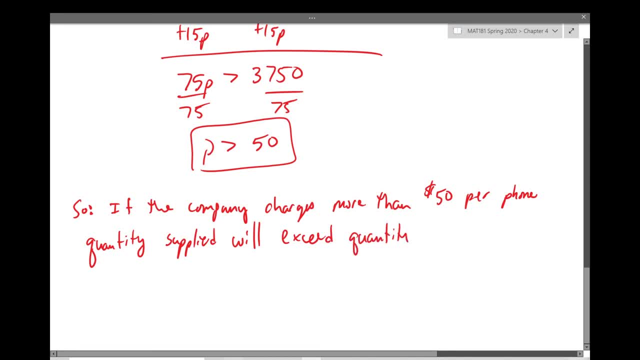 AMP: quantity demanded: Okay, In other words, what's going to happen here is this: If the company continuously increases the price above $50,, then people will no longer buy that product because they will feel as though it's too expensive and therefore the product is left on the shelves.